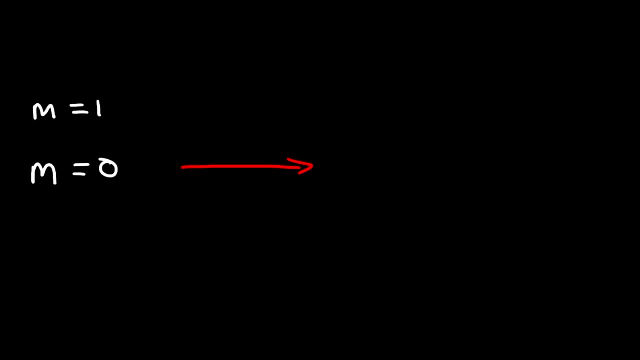 Now, if we have a slope of 1, we have a line that's going up at a 45 degree angle, And if the slope is 2, it's going to go up at a higher angle. Now, if the slope is negative- 1,- it's going to go down at an angle of 45 degrees. 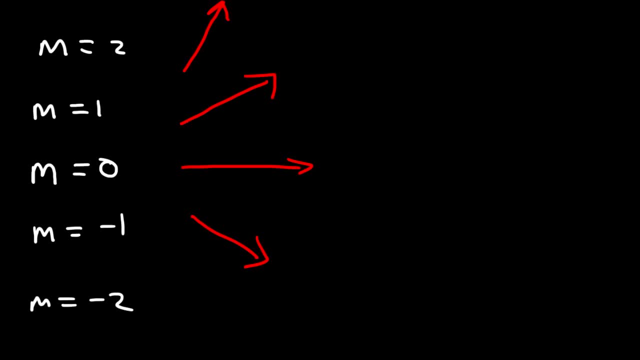 And if it's negative 2, even more so. Now, what about if the slope is very large? if it's a high number, Then you're going to have a vertical line, Or if it's undefined, you still will have a vertical line. 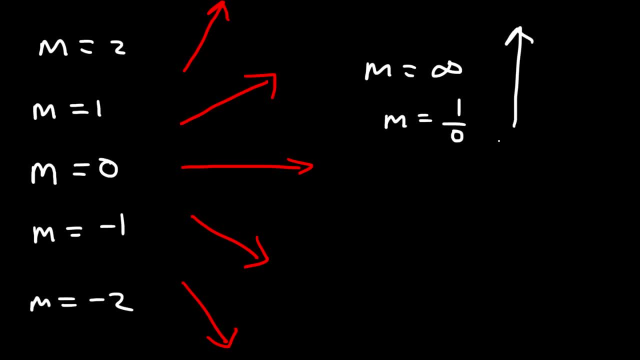 So these are some things that you want to keep in mind when drawing a slope field. So let's start with a practice problem. Let's say we have the differential equation y' is equal to x. Go ahead and draw the slope field that corresponds to this equation. 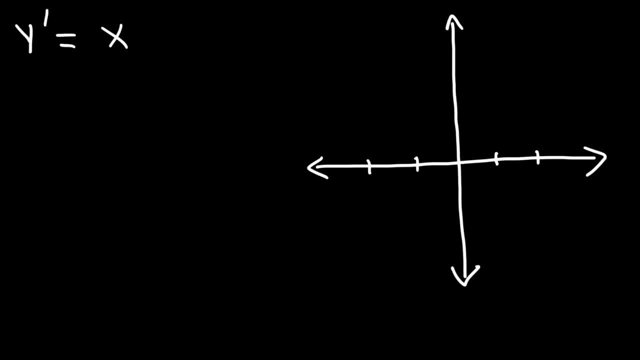 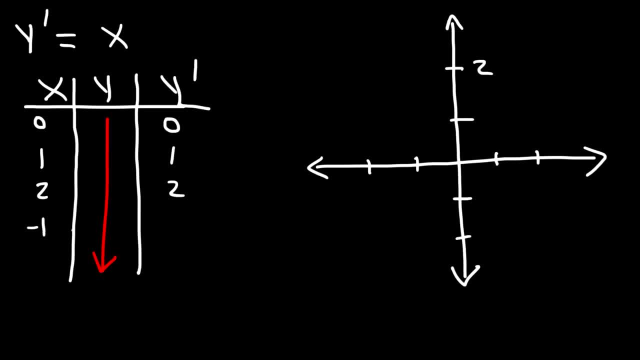 When x is 1,, that's going to be 1, and so forth. So how can we plot this? What does it mean? So when x is 0,, the slope is 0.. y' gives us the slope values. 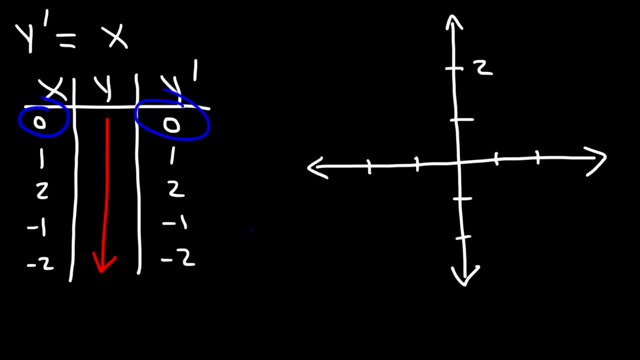 So x is 0 at the origin. So we're going to draw- I'm not sure what just happened there, but We're going to draw- a horizontal line at 0.. Now we're going to draw a horizontal line at 0.. 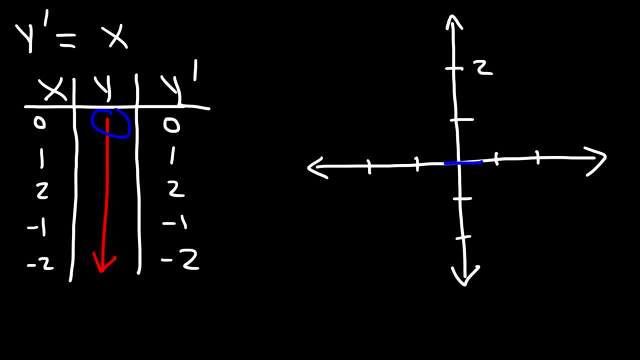 y could be anything. y could be 1,, 2,, 3,, 4, 5.. So, since y', does it depend on y anywhere where x is 0, we're going to have a slope of 0.. 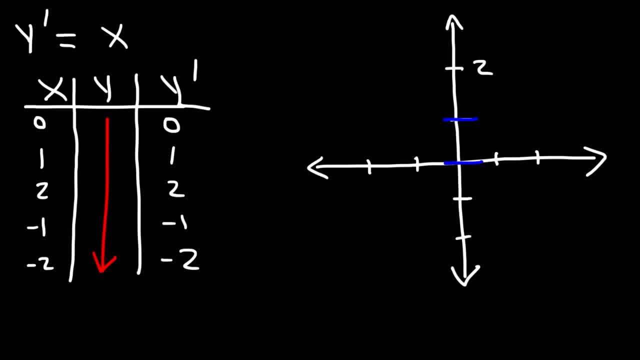 So at this point, x is 0 as well. That's the point 0, 1.. And at 0, 2, x is still 0, so the slope is 0.. So whether we go up or down, the slope will be the same. 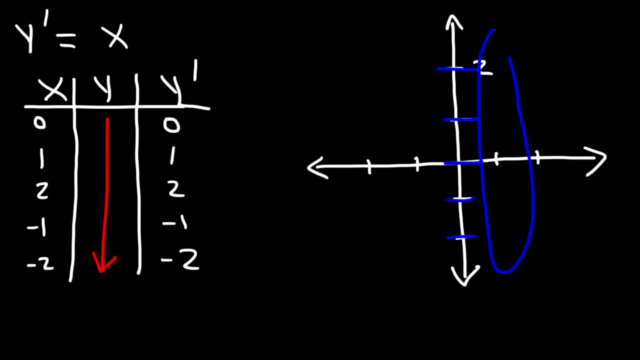 Now, when x is 1,, which is anywhere in this region, the slope is 1.. So now we need to draw a line with a slope of 1.. And then, when x is 2,, the slope is going to be 2.. 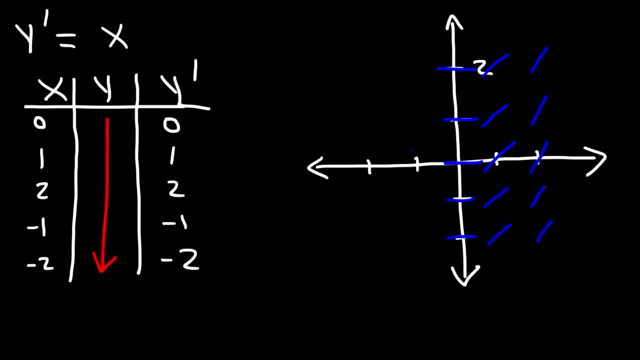 Now on the left side, when x is negative 1, the slope is negative 1.. So we're going to draw a line with a slope of 1.. And when x is negative 2, the slope will be negative 2.. 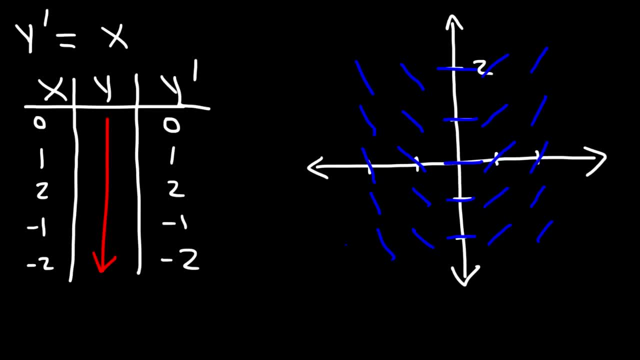 And so this is the slope field that we have for this example. Now, if we draw a line, we can get one of the solution curves, And so we can see that the general solution has a parabolic shape. Now let's solve the differential equation. 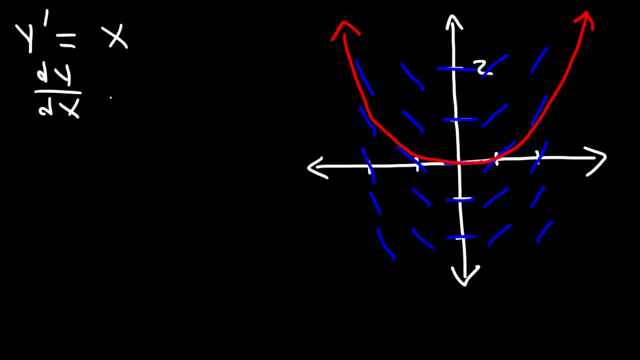 y' is basically dy over dx. Now let's separate the variables. So let's multiply both sides by dx, So we have dy is equal to xdx. Now let's find the antiderivative of both sides. The antiderivative of dy is y. 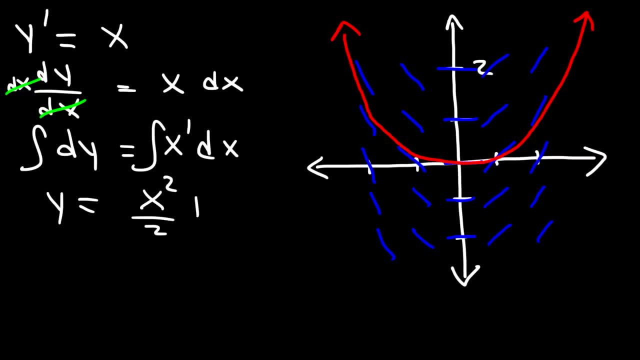 and the antiderivative of x is x squared over 2, and then plus some constancy, So we can see that 1 half x squared has a parabolic shape. It opens upward, which is in harmony with this graph. So the slope field can give you a good idea. 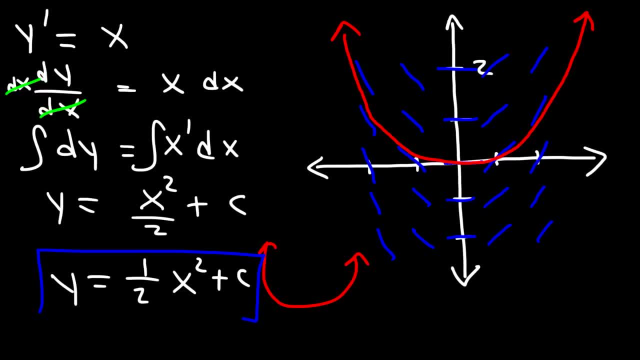 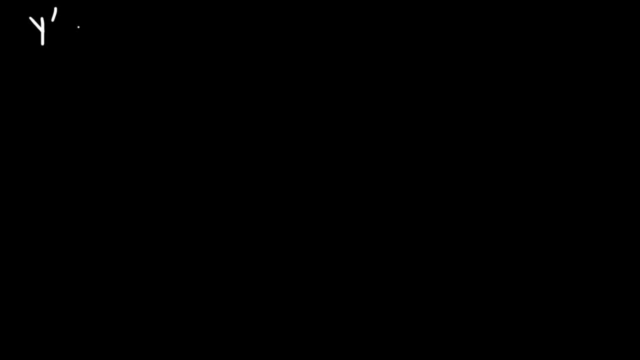 of what the shape of the solution to the equation should be. Now let's work on another simple example. So let's say y' is equal to y. Go ahead and plot the slope field that corresponds to that equation. So let's make a table. 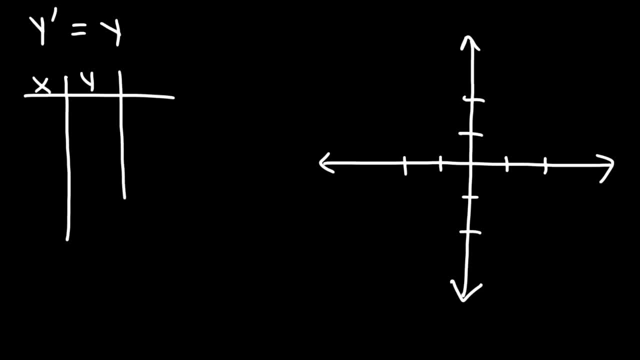 So notice that y' does not depend on x, So we don't need to put anything in that column. So when y is 0, y' is 0. So y is 0 anywhere along the x-axis, So at every point. 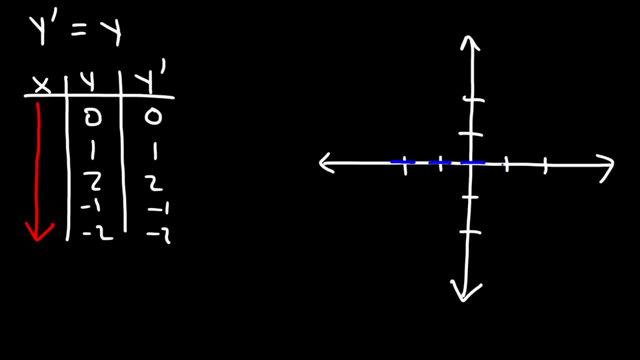 we're going to have a horizontal line. Now, when y is 1,, which is anywhere in this region, the slope will be 1.. And when y is 2,, the slope will be 2.. And then when y is negative, 1,. 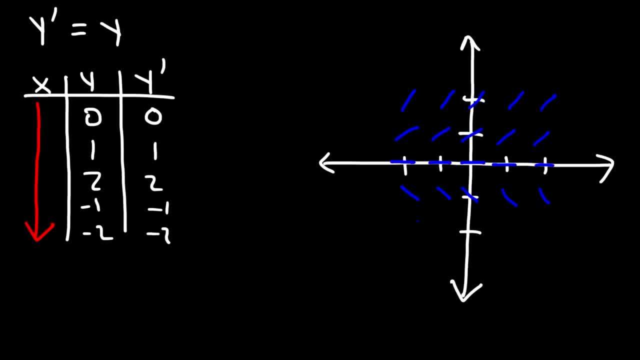 the slope is negative 1.. And then it's going to be negative 2.. So to plot the solution of the differential equation, it should look something like this: It appears to be going in that direction And that looks like an exponential function. 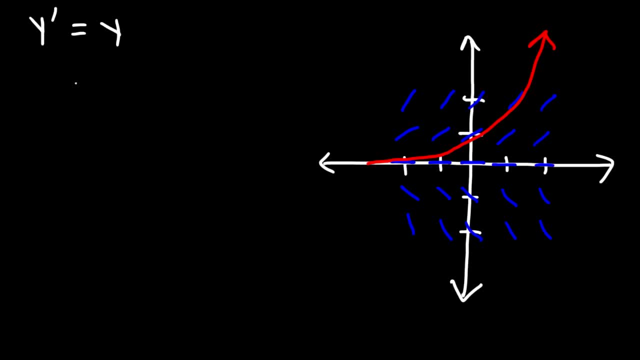 Now let's go ahead and solve this equation. So let's replace y' with dy over dx And, just like before, we're going to multiply both sides by dx, So we're going to have: dy is equal to y times dx. 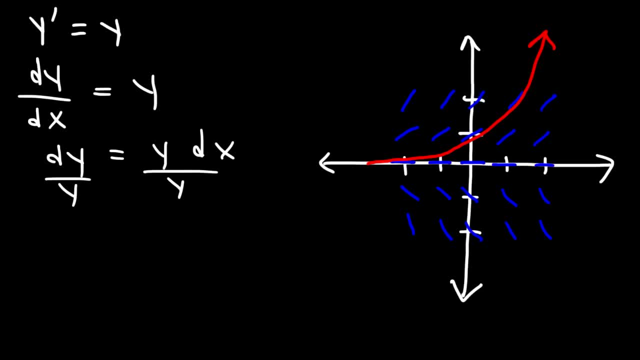 And then divide both sides by y. So on the left side we have 1 over y, and dy is equal to dx on the right side. So now we can find the antiderivative of both sides. The integral of 1 over y is l and y. 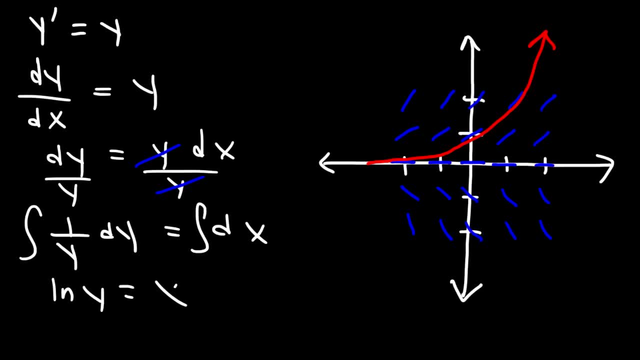 And the antiderivative of dx or 1dx is x plus c. So now we're going to put both sides of the equation on the exponent of e. So we're going to have e raised to the l and y is equal to e raised to the x plus c. 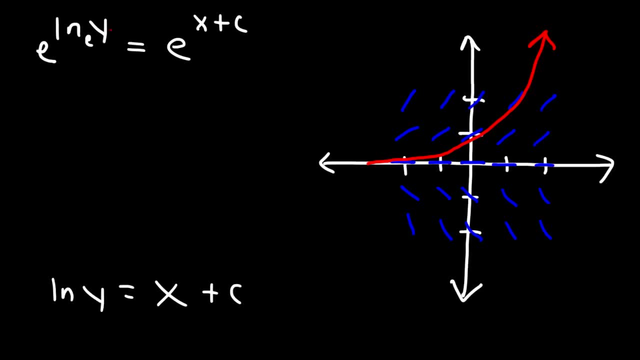 Now e to the l and y. the base is e and so this simplifies to just y And e to the x plus c. Let's say, if you have x to the 7, you can write that as x to the 3 plus 4,. 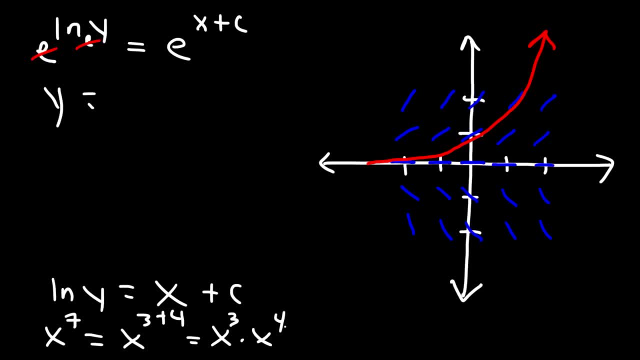 because 7 is 3 plus 4.. And then you can separate it into two parts. That's x cubed times x to the 4th, So e to the x plus c can be written as e to the x times e to the c. 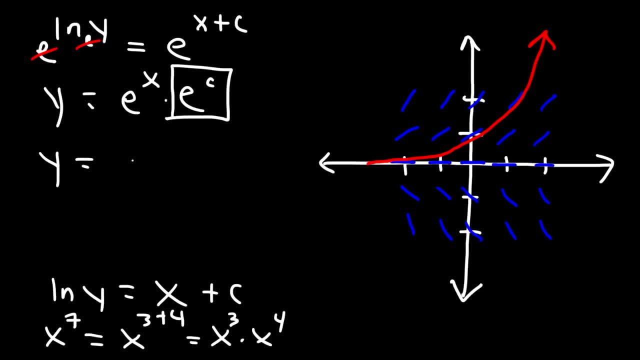 And e to the c is a constant, So we can replace that whole thing with a constant. So the solution is going to be: y is equal to 7, c, e to the x, And exponential functions have the general shape. that looks something like that: 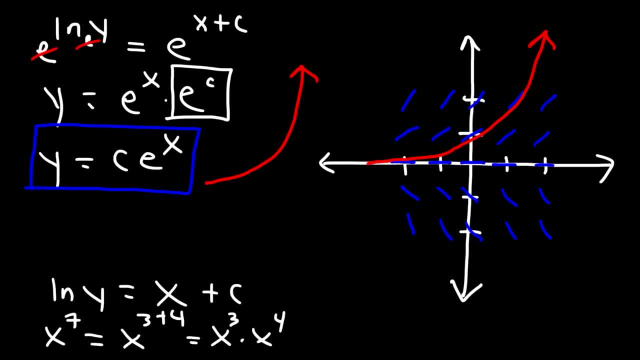 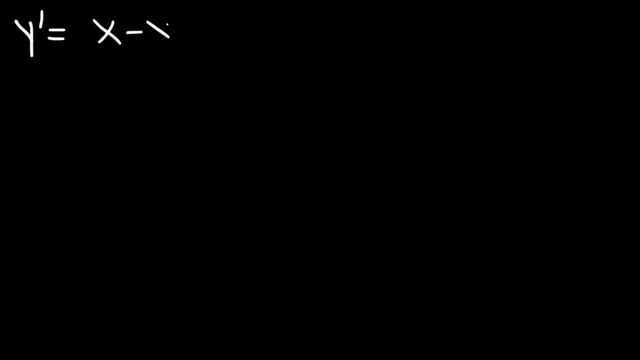 which is what we have in this example. So once again, the slope field. it gives you a good shape of the solution to the differential equation. Now let's move on to our next example, where y prime is x minus y. So this time, 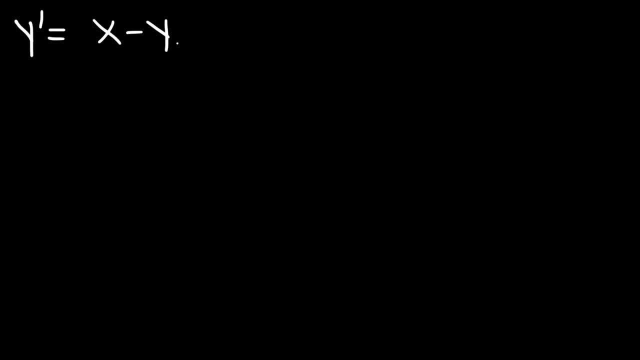 y prime depends on two variables as opposed to one in the last two examples. So this is going to be a little bit harder to graph, But we're going to follow the same process. So lets start with zero. So lets start with 0.. 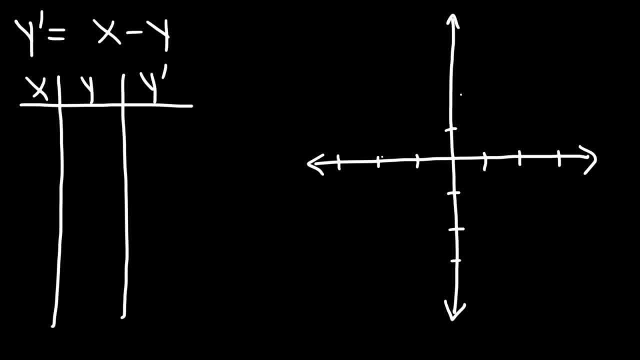 When x is 0 and y is 0,, the slope is going to be 0.. So let's find out that when y is 0, and y is 1,, the slope is going to be 0.. When y is 0,. 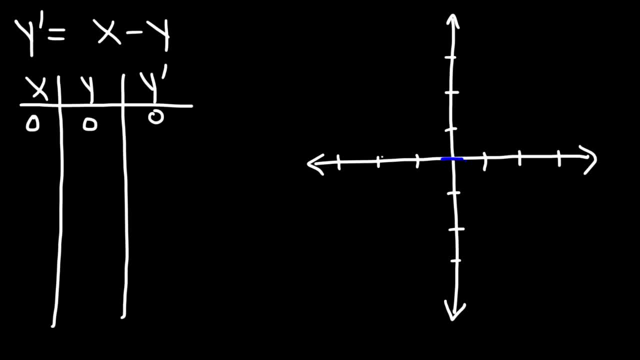 the slope is going to be 0.. The slope of x is 0.. The slope of y is 0.. Now notice that when x is 1 and y is 1, the slope will also be 0. There's a little bit of a difference. 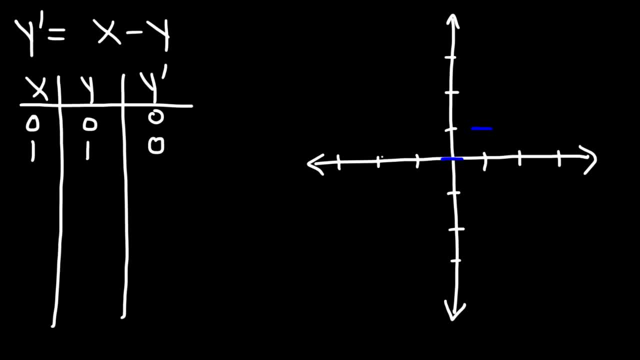 between this one and the first one. So when x is 2 and y is 2, the slope is zero. 2 minus 2 will be 0.. When y is 2, the slope is 2.. So notice the pattern that's forming here. 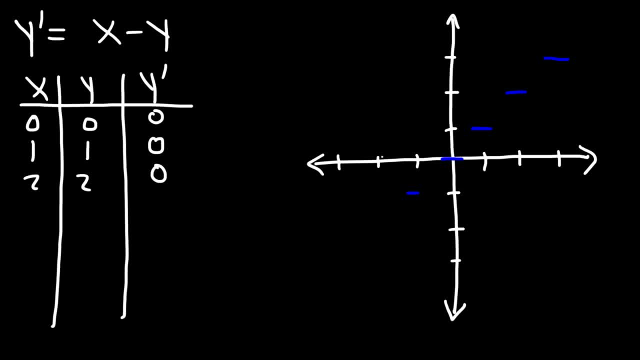 So continuing the pattern. anytime x and y have the same value, the slope will be 0. And you want to look for patterns because it helps you to quickly plot the slope field. Now what is the next pattern that we can identify? So what about when x is 1 and y is 0?? 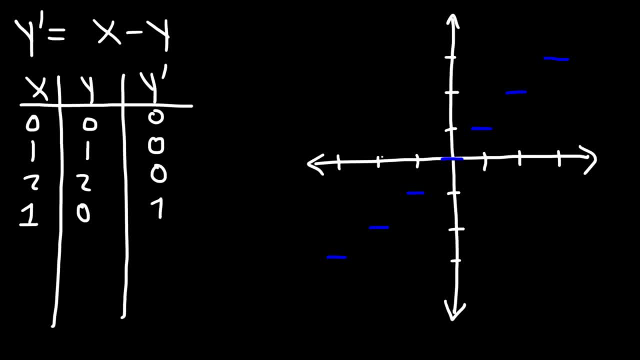 When x is 1 unit higher than y, 1 minus 0 will be 1.. So we're going to have a slope of 1 at this point. Now what about when x is 2 and y is 1? 2 minus 1 is still 1.. 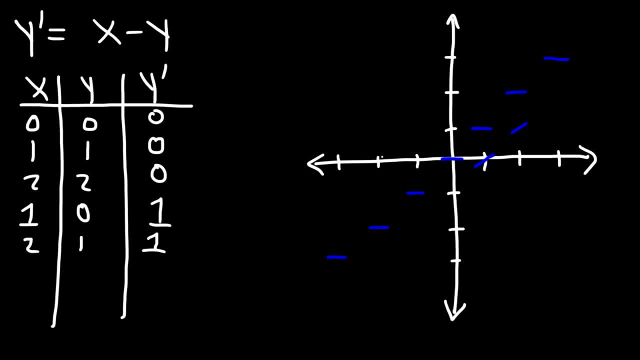 And so the point 2 comma 1 is here, And then the next point 3 comma 2, 3 minus 2 is 1.. Now, if we go backwards, this will take us to the point 0, negative 1.. 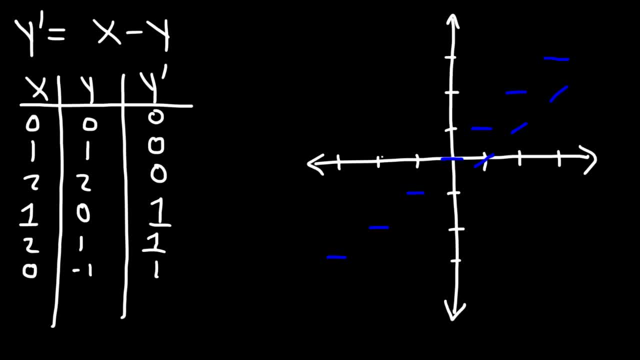 And 0 minus Negative 1 is still positive 1.. So then this point where x is negative 1 and y is negative 2, that's still going to give us a slope of 1.. And so the pattern will continue. 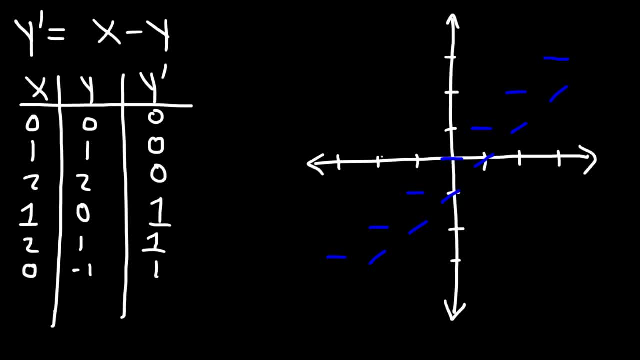 Now let's try the next point. Let's try 2 comma 0. So 2 minus 0 is 2.. So the slope here will be 2.. And then, if we try the next point, Let's say 3, 1.. 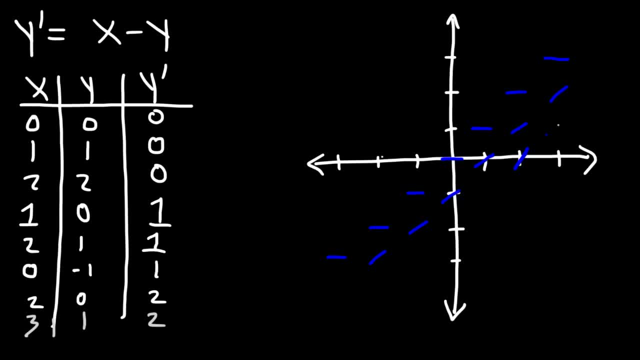 3 minus 1 is still 2.. So we can see the same thing. that's happening Now. what about this point? Let's make a new table. So, when x is 0 and y is 1, 0 minus 1 is negative 1.. 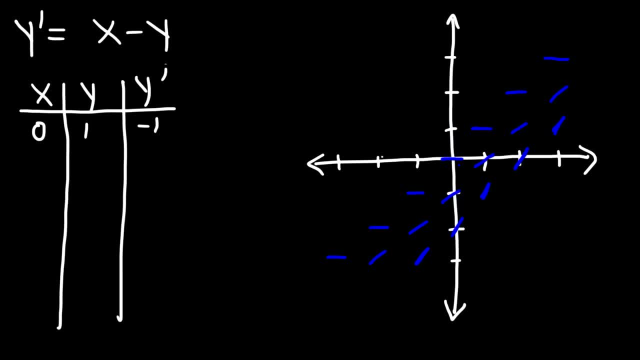 So this is going to look like this. So this point here should be the same thing if it follows the pattern. So when x is 1 and y is 2, 1 minus 2 is still negative 1.. So now that 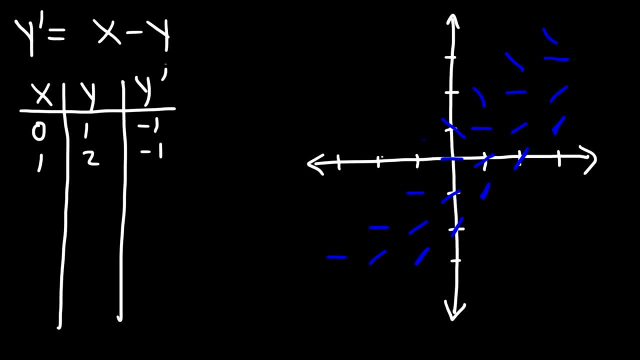 Now that a pattern has emerged, we can just continue the pattern. Now let's focus on this point. When x is 0 and y is 2.. So 0 minus 2 is negative 2.. And so this is going to look like that. 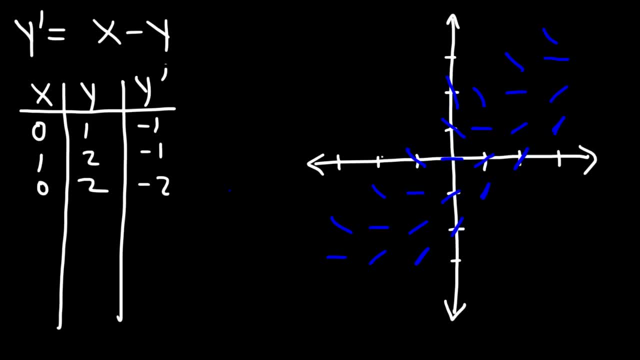 And then I imagine at this point it should be the same. That's when x is 1 and y is 3.. 1 minus 3 is still negative 2.. And then after that we can see that the slope is becoming more negative. 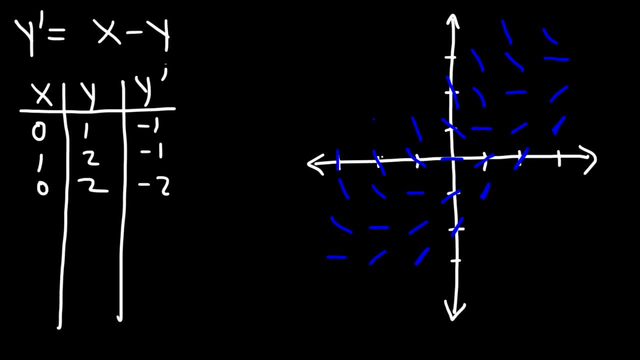 So the next one should look something like this: It's going to be almost vertical. We could just fill it in at this point And it's not going to change Now, continuing this trend, If we plug in this point where x is 3 and y is 0,, the slope is going to be 3.. 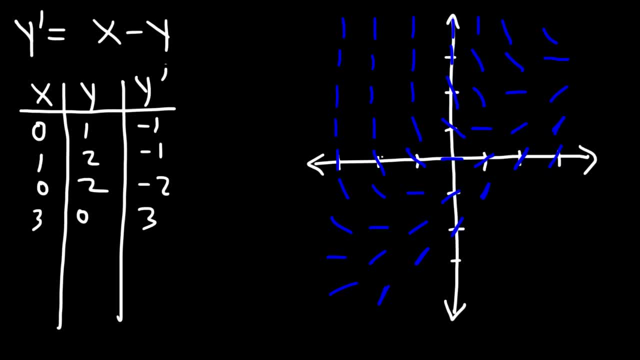 So it's going to be almost vertical at that point. So, And then after that we could just draw vertical lines, Because that's going to be the trend in this region. So now we have a good estimate of the slope field that corresponds to this differential equation. 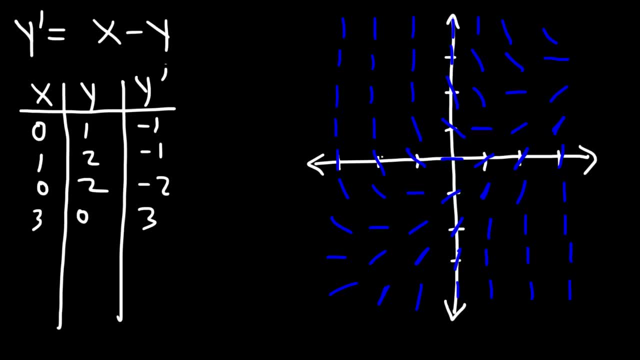 And it turns out that the solution, or at least one solution that we can draw, is this straight line here. So notice that one of the solutions to this equation is a linear equation. Now, if you want to know how to solve this differential equation, how to integrate it, 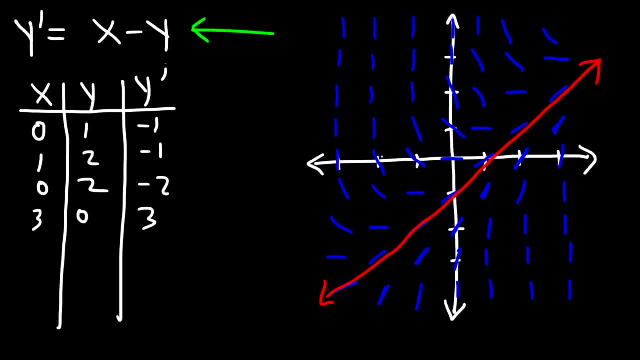 there's another video I have on YouTube entitled First Order Linear Differential Equations. So if you watch that video, you'll be able to see how you can solve that differential equation, And so what you need to do is put it in the appropriate form. 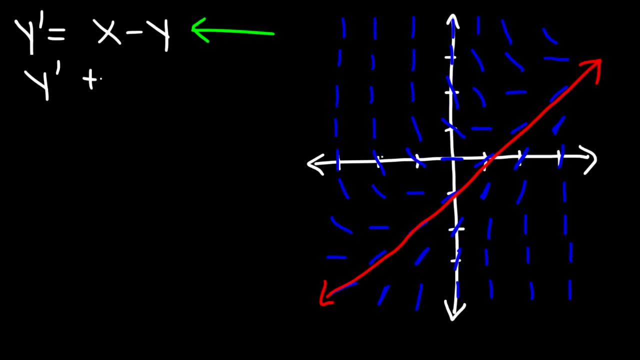 Which is going to be y. prime plus y is equal to x. Now, once it's in standard form, the video will show you what to do from this point. So I'm going to give you the solution to the differential equation, and you can verify it that it is indeed a solution. 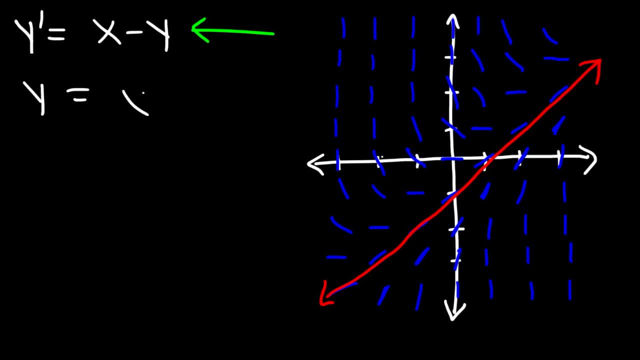 So the solution is: y is equal to x minus one, And you can see it here, This graph, you can see the y intercept is negative one. So that point is zero, negative one. And if you plug in zero for x, you're going to get negative one for y. 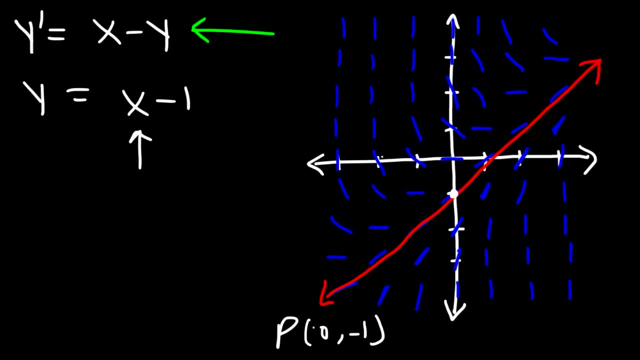 Zero minus one is negative one, So the solution passes through this point. Now we can verify that this is indeed the solution to this differential equation. If we calculate y prime by taking the first derivative of this function, the derivative of x minus one is going to be one. 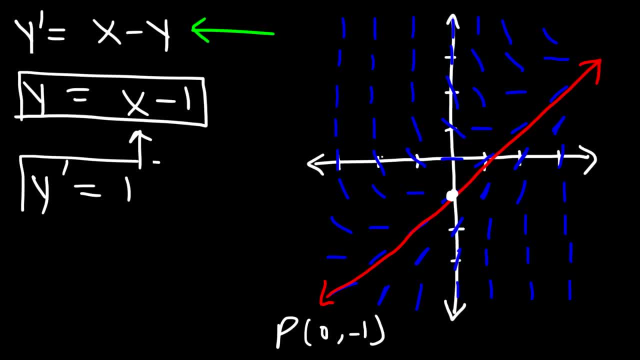 And the derivative of negative one is zero. So this is y prime. Y prime is one. So let's plug in y prime And y into the differential equation, So y prime is one, And then we have x minus y, where y is x minus one. 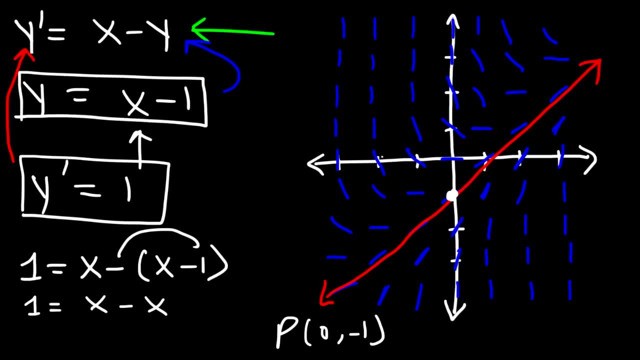 So this is going to be x minus x, And then negative times. negative one is plus one. These two will cancel, And so we can see one is equal to one. So therefore, this line in red represents the solution to the differential equation, which is: y is equal to x minus 1.. 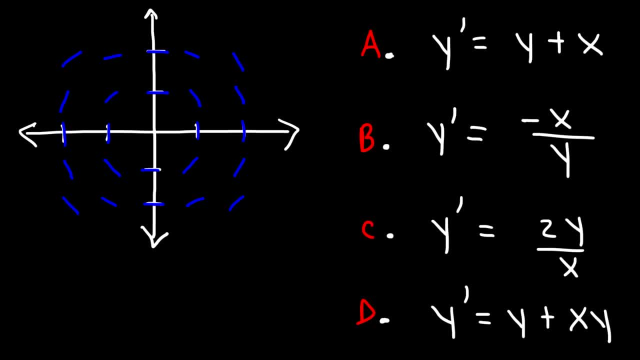 Now here's a multiple choice problem and we're given a graph of the slope field and we need to match it to the appropriate equation. Now what you need to do is pick a point and see if that point works for each equation. So let's focus on this point At that point. 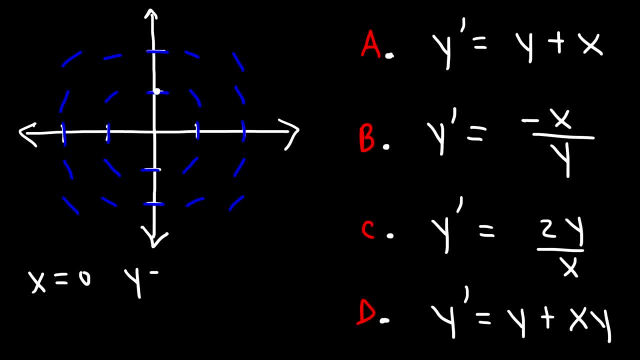 x is 0,, y is 1, and the slope? notice that we have a horizontal blue line. so y prime, the slope has to be 0.. Now let's look at answer choice A. If we plug in these values, will y prime be 0?? So y plus x, that's going to be 1 plus 0.. 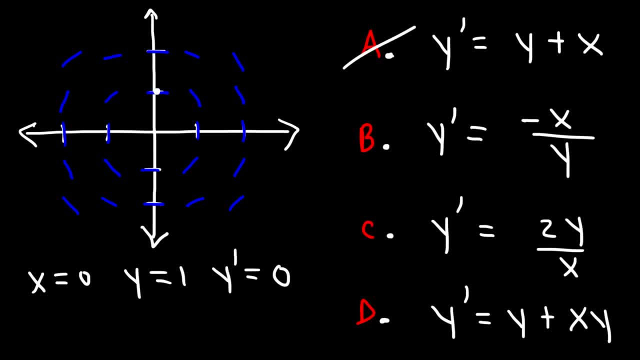 1 plus 0 is 1.. It doesn't equal 0, so we can eliminate answer choice A. Now you want to eliminate every answer until you get the right answer. Now let's move on to answer choice B. 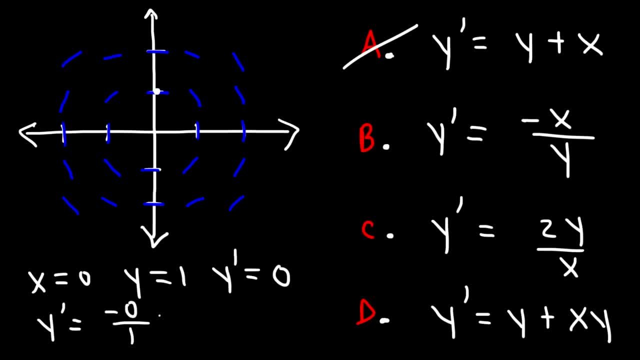 So x is 0, y is 1.. Negative 0 divided by 1 is 0.. So far B is okay. It works for that point, so we won't eliminate that answer. Now let's move on to part C. 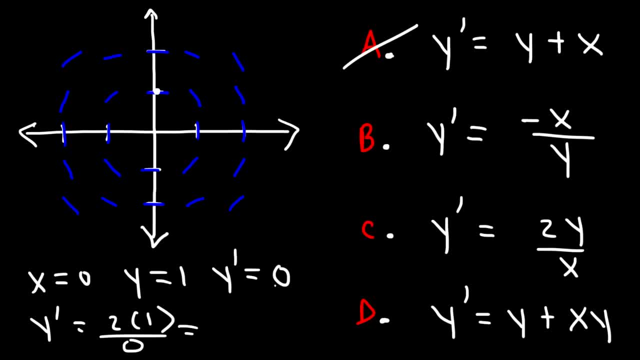 y is 1, x is 0. So this is 2 over 0, so it's undefined, which means we should have a vertical tangent, Not a horizontal line. So we can eliminate answer choice C. Now, moving on to answer choice D. 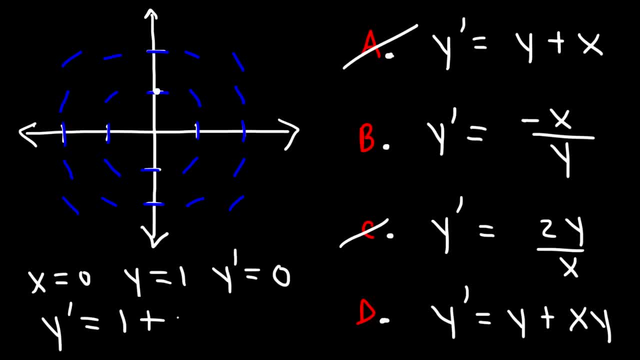 Let's plug in the same points. So y is 1, x is 0. And so this is going to be 1 plus 0, which is 1.. So we need a slope of 0, not 1.. So that would correlate to a blue line. 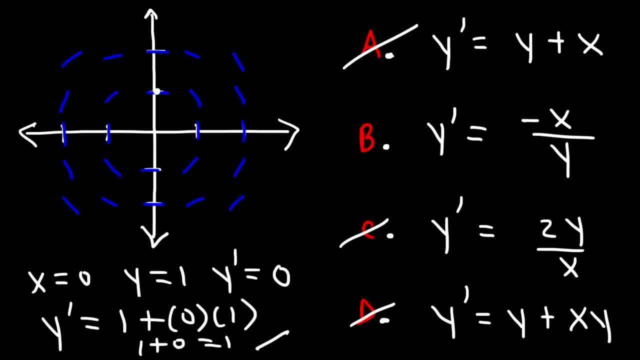 That looks like that. So D can be eliminated. So the right answer is B. That is the differential equation that corresponds to this slope field, And so you just got to plug in points and then you can match it with the right equation. 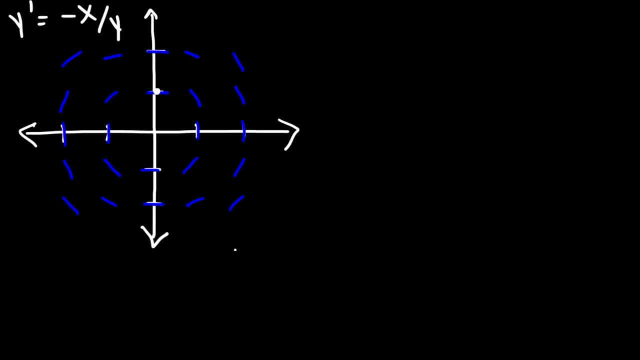 Now, looking at the slope field, what type of graph do we have? Notice that we have the shape of a circle. Now, you can have a big circle or you can have a small circle, but the general shape is a circle. 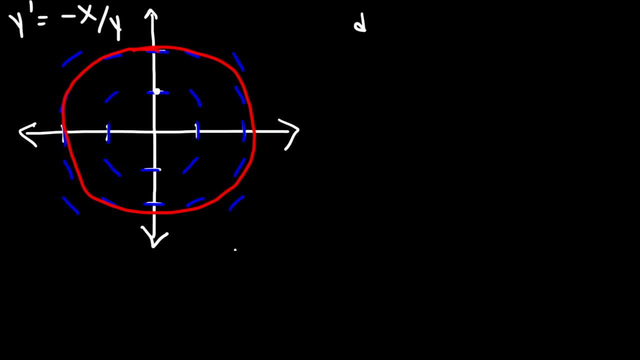 Now let's solve the differential equation. So let's replace y prime with dy over dx, And so that's equal to negative x over y. And let's cross multiply, So we're going to have y times dy, And that's equal to negative x. 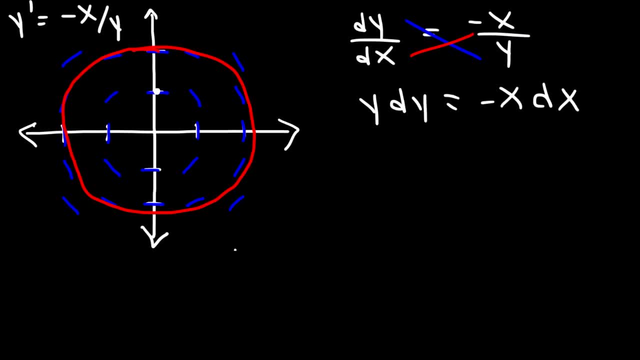 And that's equal to negative x times dx. So now let's integrate both sides. The antiderivative of y is y squared over 2.. And the antiderivative of negative x is negative x squared over 2 plus c. Now I'm going to take this term and move it to that side. 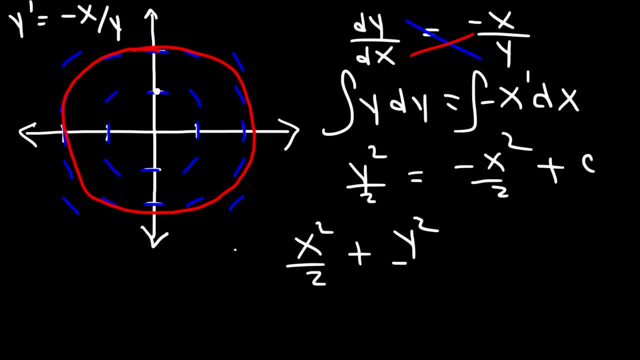 So I have x squared over 2 plus y squared over 2.. That's equal to c. Now let's multiply both sides of the equation by 2.. So the 2 is equal to 2.. The 2s will cancel. 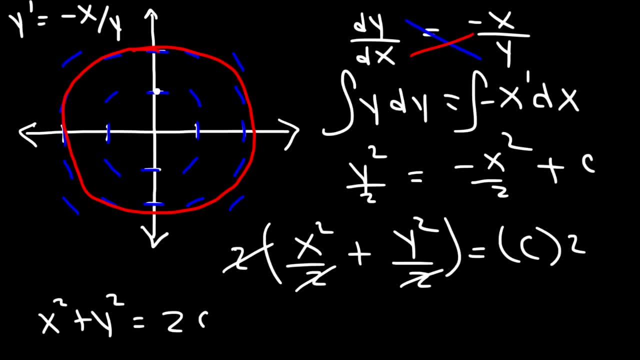 And so we'll be left with x squared plus y squared, which is equal to 2c. Now, 2c is a constant, so we could just replace that with c. So this is the general solution of the differential equation. 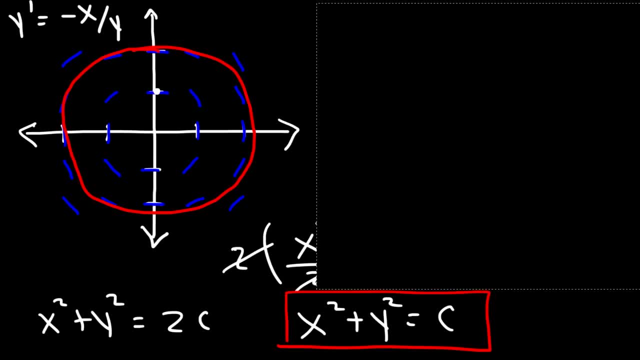 Now, x squared plus y squared equals c. What equation does that look like, so to speak? So notice that. Notice that this equation is identical to the equation of a circle, which is x squared plus y squared, and that's equal to r squared. 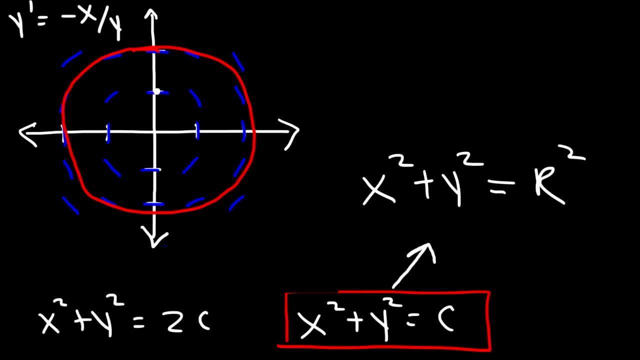 And r represents the radius of a circle, which is a constant for a specific circle, And so for this circle we can see that r is equal to 2.. So for that red line that I drew, if r is 2, the solution of that particular equation will be: x squared plus y squared is equal to 4..